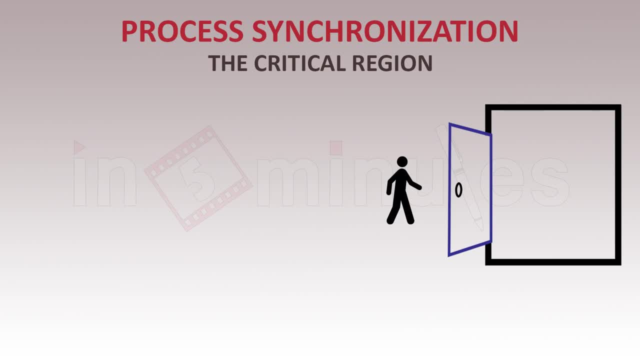 there is a room- may be a fresh room- in which there is a queue of n people standing. Now, the room can be used only by one person at a time. Let's number them. This person- A, let's say this- is B, C, D and E. Considering that A has already gained access, others are in. 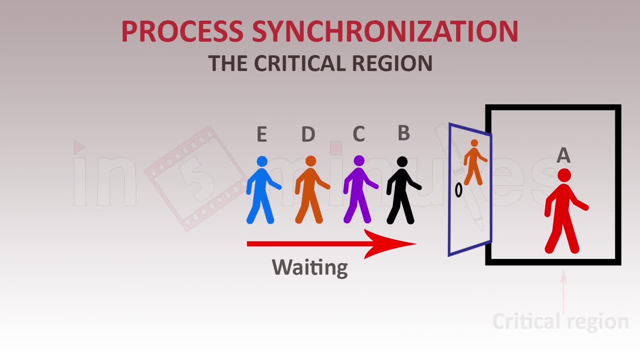 waiting and A is within the critical region or a critical section, The moment A finishes its job. what would happen? A would simply come out of it. Then from the waiting queue, depending on some algorithm, Mr B enters the system. Now C, D and E are waiting. The moment B will finish its job, again the same thing would 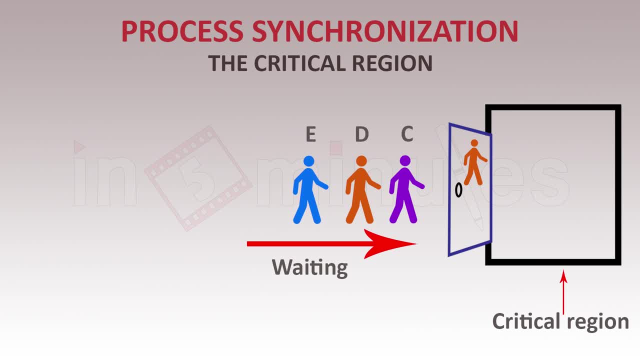 happen: B would go off and probably the next one, C, gets in and the system would repeat. So basic idea over here is to understand the critical region noon. over here is a specialised reason which can be accessed, one at a time manner. The term is known as mutual exclusion. This can be used for several things. now, If you practically 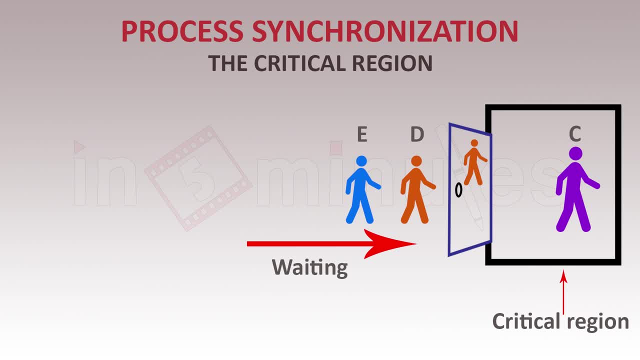 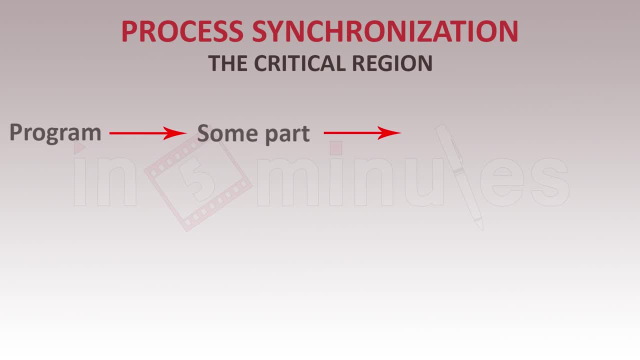 try to understand how critical region and why critical region. let's try to PUT it: EVERY program will have some part which is needed to access in mutual exclusive manner. Now this some part might end up. Now this some part may refer to file access, database access can be some variable access. 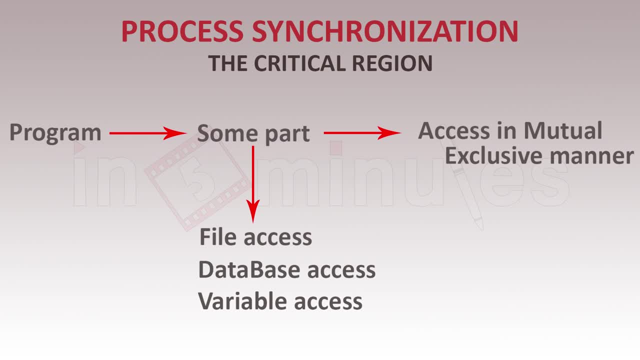 Now, this kind of access would require special attention. Why Maybe, when a program is accessing a particular file, maybe that file is used by 10 other processes. By this process changing this particular file- X, Y and Z would be affected, which we don't want. 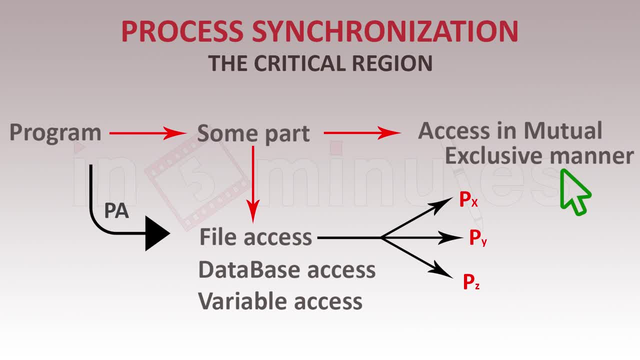 Hence process A would require mutual exclusion so that only it can access, modify the file and then later on others can access this information. Similar can be seen or understood for the database access or for the variable access. We don't want anybody.